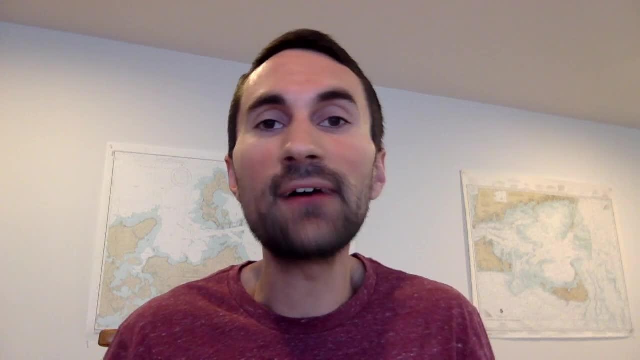 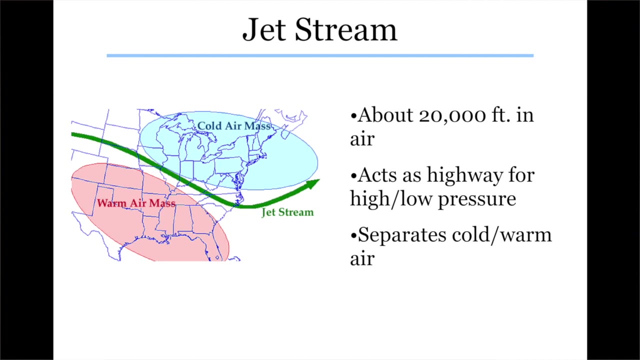 way high in the atmosphere. We're talking 20,, 30,000 feet in the sky. That's the jet stream. The jet stream is basically a fast moving river of air and it drives storms, in our case across the country towards New England. Now it will ebb and it flows It. 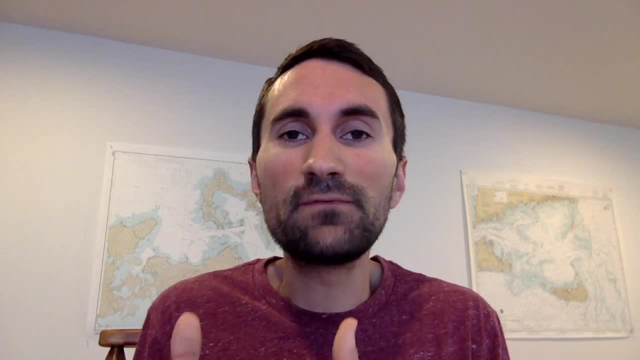 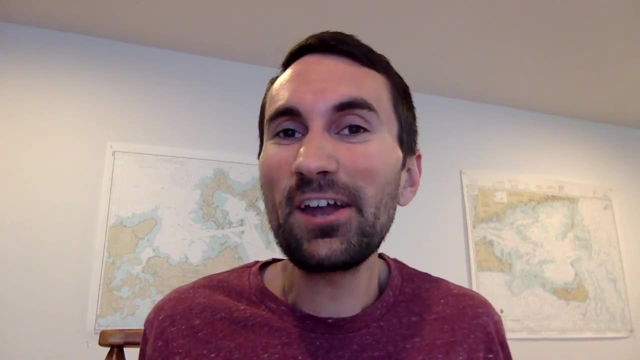 moves around, basically, but it's the storm track. This very fast moving ribbon of air way high in the sky is somewhere you've actually been, believe it or not. If you've been on an airplane, you've been in the jet stream. The storms obviously follow the jet stream, but so too. 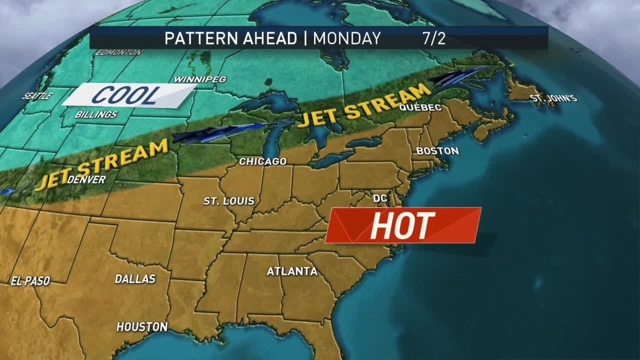 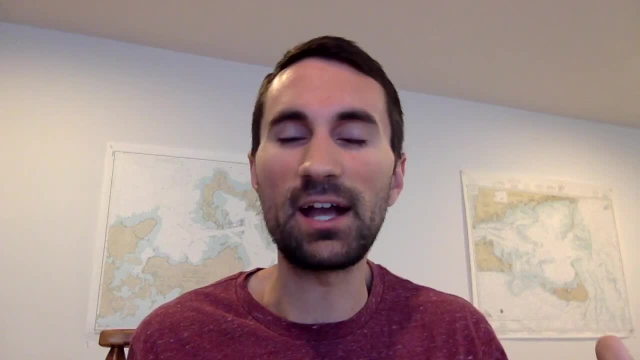 do airplanes in some cases. So think about it. The jet stream flows from west to east. It separates cold air to the north and warm air to the south. Temperatures will change as the storm track changes. Now why would a plane be in a jet stream? Might sound like. 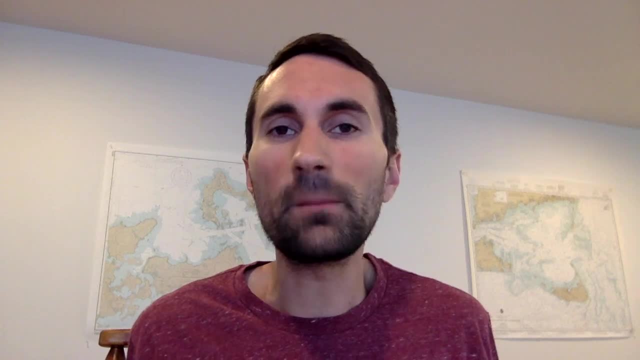 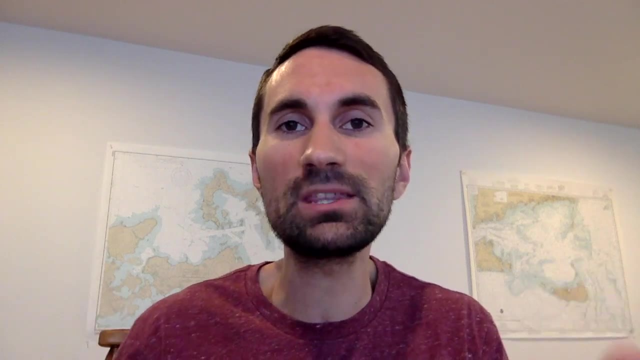 something. that's kind of weird, but it actually works to our advantage. When a pilot is flying to Boston, if you fly with the jet stream, you have this wind at your back that's pushing the plane forward and making it move much faster. By contrast, if you're flying from 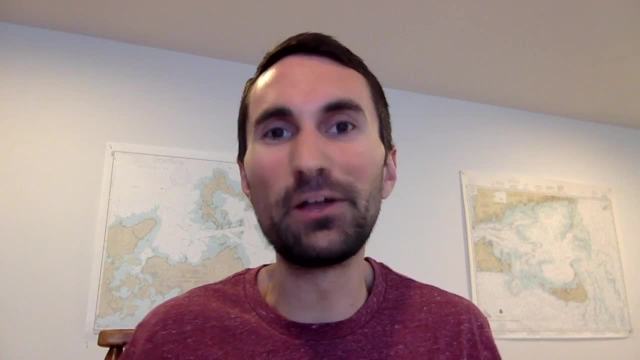 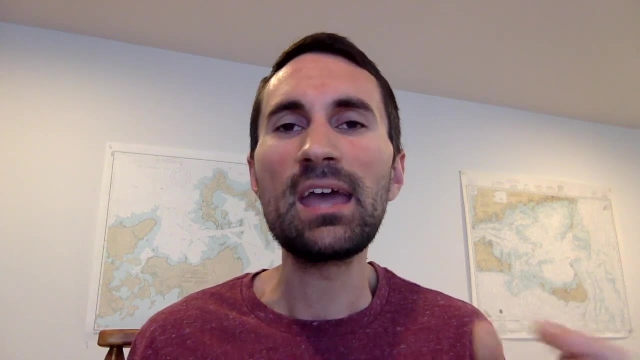 Boston to San Francisco, you might want to avoid the jet stream, because you're flowing right into that fast moving ribbon of air and it will slow you down. So just like riding a bike: if you have a wind at your back, you're going to go faster, and if you have a wind, 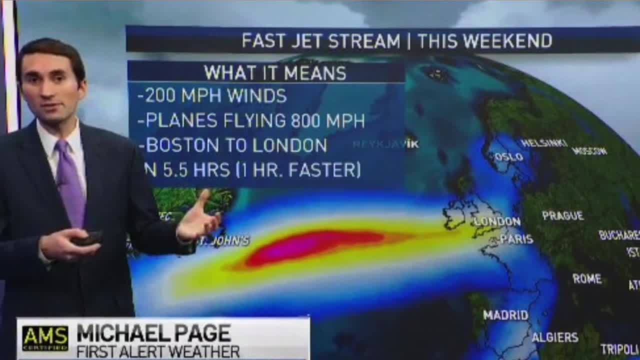 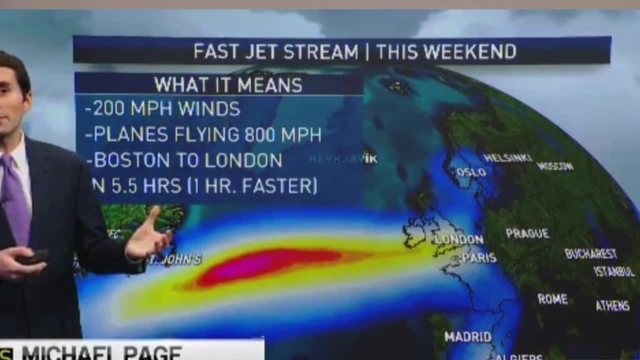 in your face. you're going to go slower Now. just a couple of weeks ago, we talked about this: how a plane from Boston to London arrived in about five hours because of a really intense jet stream over the Atlantic. That's one. 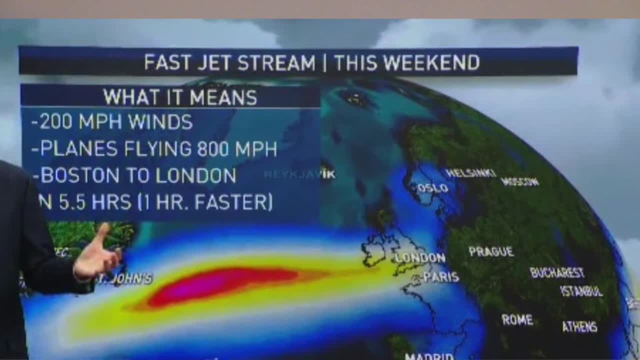 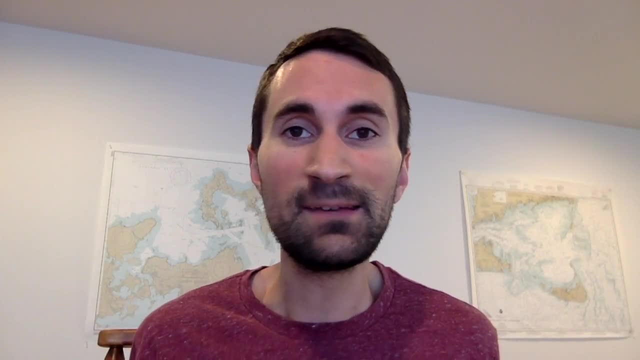 of those cases where the pilot locked in on where the jet stream is, flew with it and got to England a lot faster than he or she would have otherwise. There was also just a plane, because of this coronavirus situation, that flew from parts. 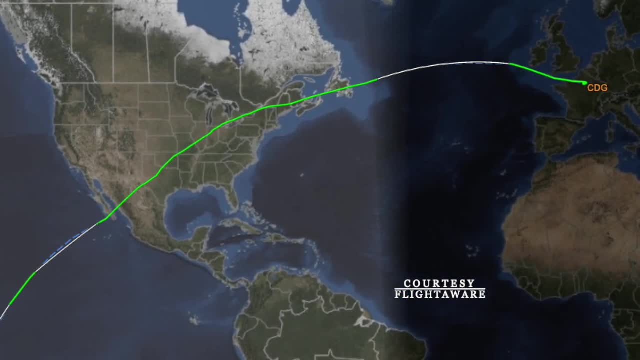 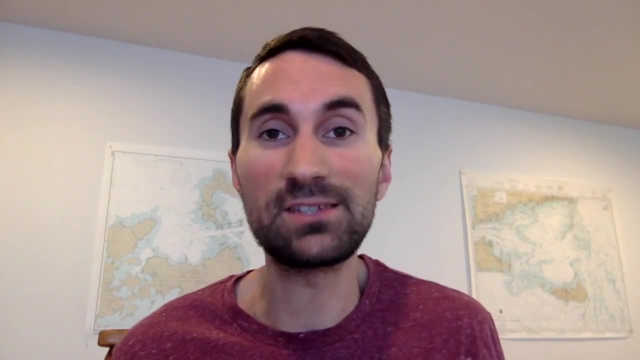 of French Polynesia all the way to Paris nonstop. That's a long flight, but the pilot was able to fly with the jet stream to make it happen, And the reason they were flying that far is because they didn't want to stop in the United States where people could be quarantined. 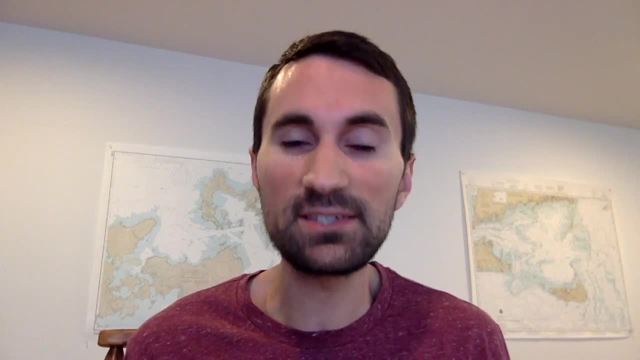 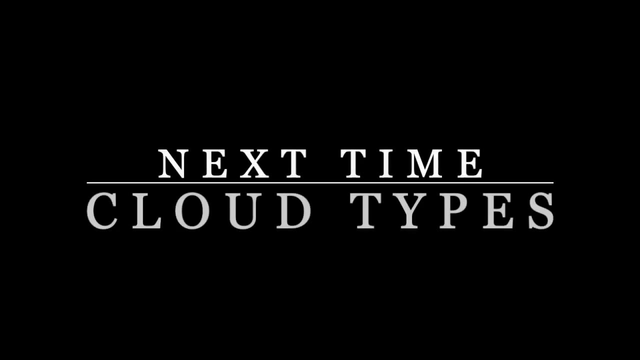 or what have you. So the jet stream is a big driver, not just in our weather, but also very helpful for pilots and anyone who flies Coming up. in our next lesson we're going to talk about the different types of clouds.